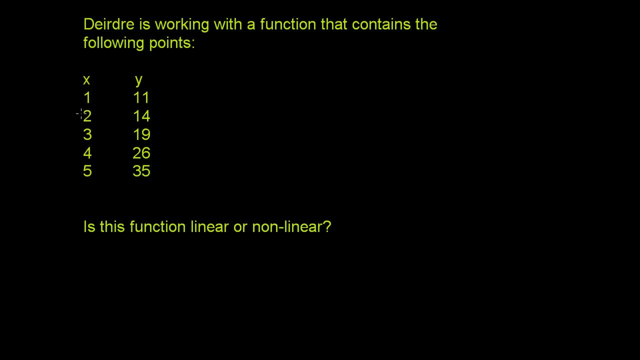 with a linear function If for each change in x- so over here- x is always changing by 1.. So since x is always changing by 1, the change in y's have to always be the same. If they're not, then we're dealing with a. 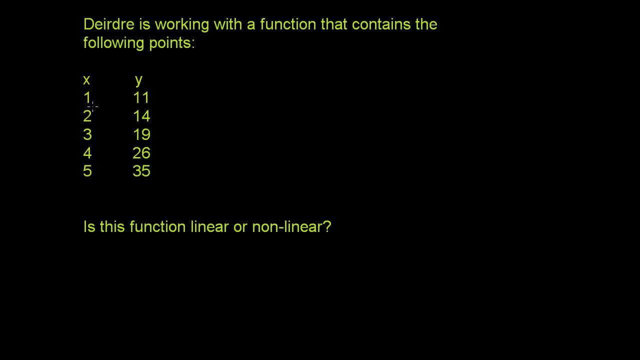 nonlinear function. We can actually show that plotting out. If the changes in x were going by different values, if this went from 1 to 2 and then 2 to 4, what you'd want to do then is divide the change in y by the change in x. 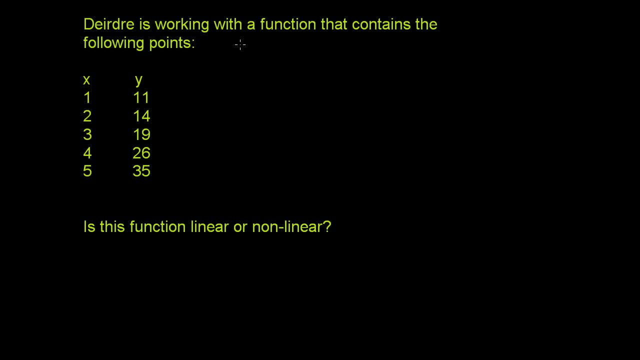 And that should always be a constant. In fact, let me write that down: Linear. if something is linear, then the change in y over the change in x always constant. Now, in this example, the change in x's are always 1.. 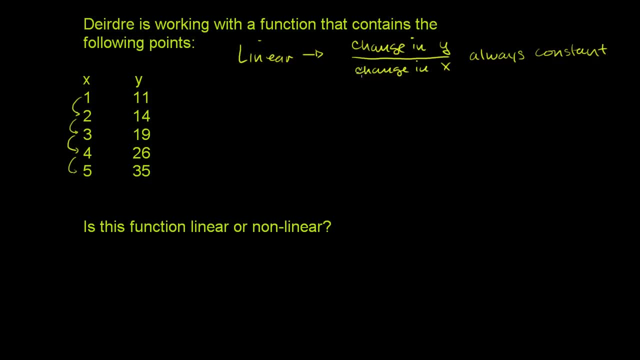 We go from 1 to 2,, 2 to 3,, 3 to 4,, 4 to 5.. So in this example, the change in x is always going to be 1.. So, in order for this function to be linear, our change in y: 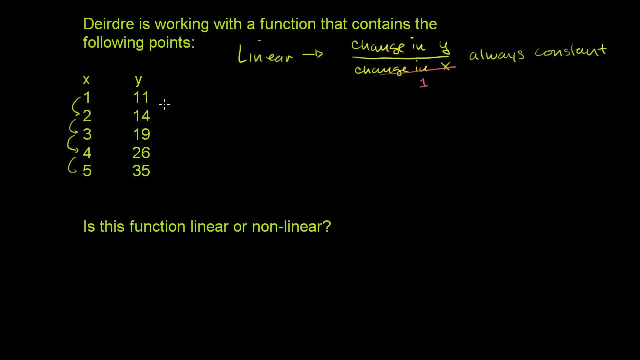 needs to be constant, because we're just going to take that and divide it by 1.. So let's see if our change in y is constant. When we go from 11 to 14, we go up by 3.. When we go from 14 to 19, we go up by 5.. 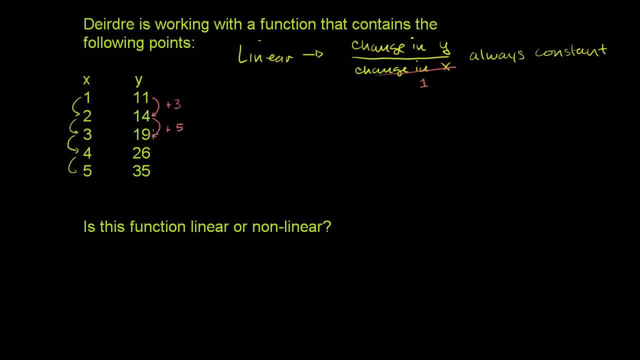 So I already see that it is not constant. We didn't go up by 3.. This time we went up by 5.. And here we go up by 7.. And here we go up by 7.. And here we're going up by 9.. 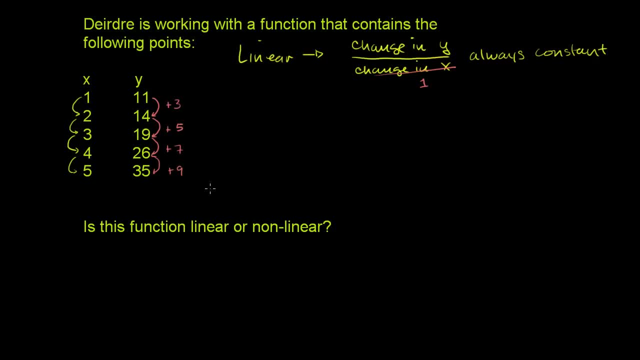 So we're actually going up by increasing amounts. So we're definitely dealing with a non-linear function And we can see that if we graph it out. I'll do a rough graph here, So let me make that my vertical axis, my y-axis. 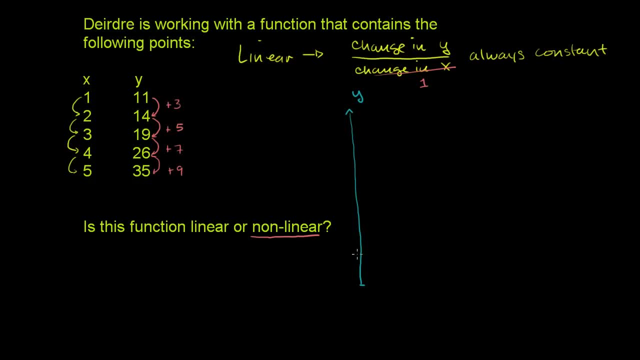 And we go all the way up to 35.. So I'll just do 10,, 20,, 30. Actually, I could do a little bit more granular than that. I could do 5,, 10,, 15,, 20,, 25,, 30, and then 35.